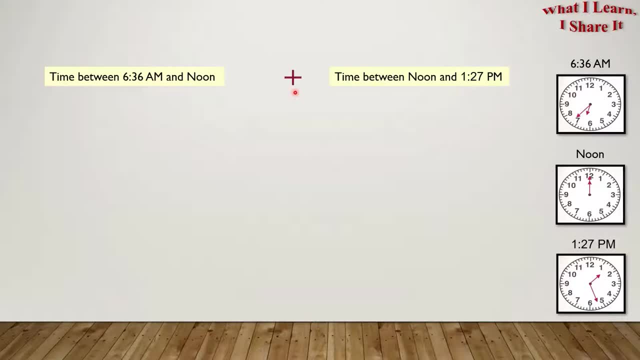 durations to get the total time duration. So let's take part 1.. Time between 6: 36 am and noon. For this we can subtract 6: 36 from 12 o'clock. So here we go. So the time between noon and 1: 27 pm is 1 hour. 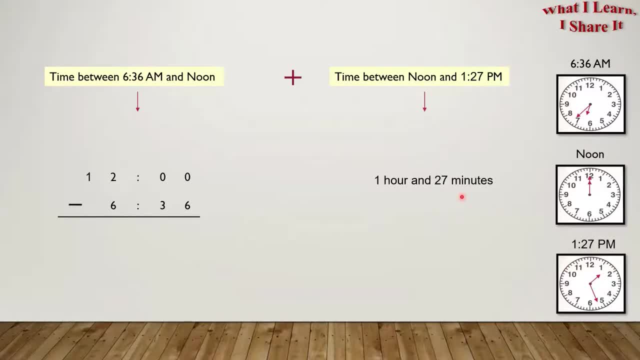 and 27 minutes. This was pretty easy because noon is at 12 o'clock and it doesn't go to 13 o'clock. So what I did is: from 12 o'clock I added 1 hour, which would be 1 o'clock, and then 27 minutes, which would be 1 hour and 27. 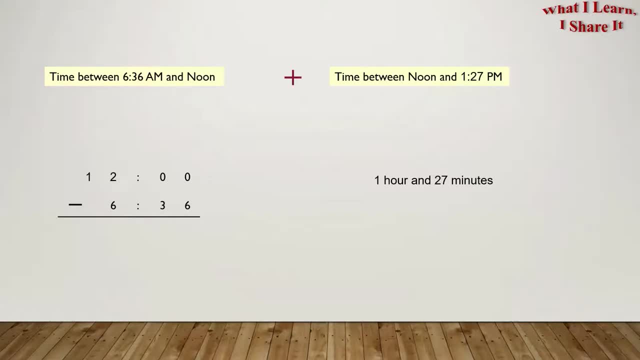 minutes. So there is 12 o'clock minus 6, 36.. But as you see, on the minute side, 36 minutes cannot be subtracted from 0 minutes, So we will have to borrow from the hours. But what will we get? We will get 1 full hour, But 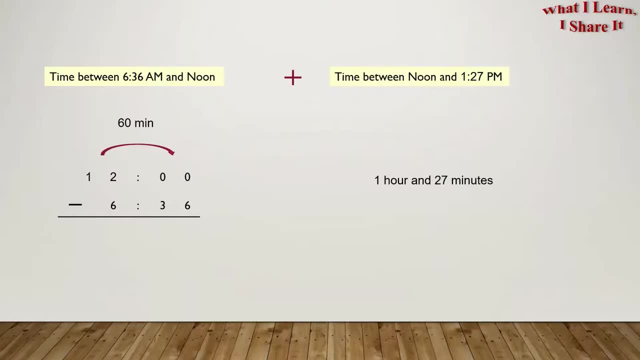 1 hour is also 60 minutes. So, instead of 12 hours, we are going to write 11 hours, and instead of 12 hours, we are going to write 11 hours, and instead of 12 hours, we are going to write 12 hours. 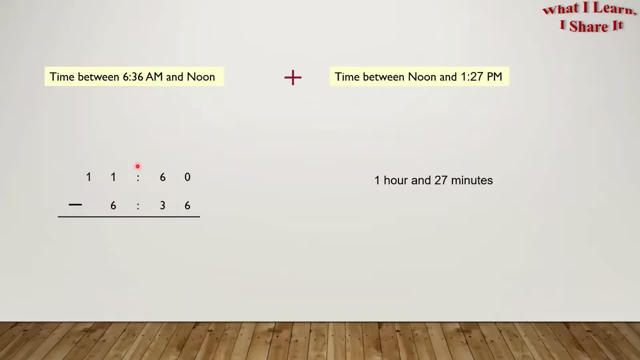 So now we have 16 minutes. You see that we get 1 half hour, which is a touchdown, But we are going to try and subtract 2 of these 12 hours. So, instead of 12 hours and 3 minutes, we are going to do 16 minutes. So what we are going to do is we are going to 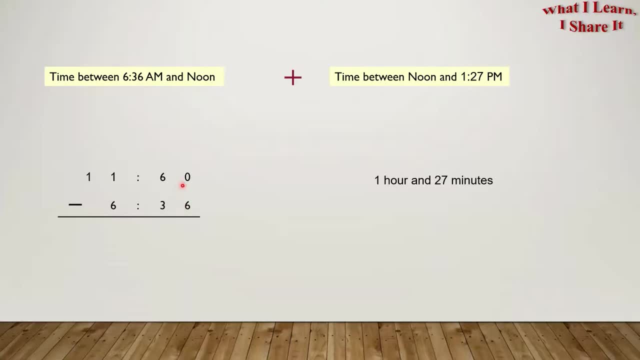 subtract 10 to the power of 10, which I believe is in Live Committee, and then we are going to subtract 30. We are going to subtract 70 here, and then we are gonna subtract an він, from which means we are going to subtract 1,, 2, and 3.. So the sum 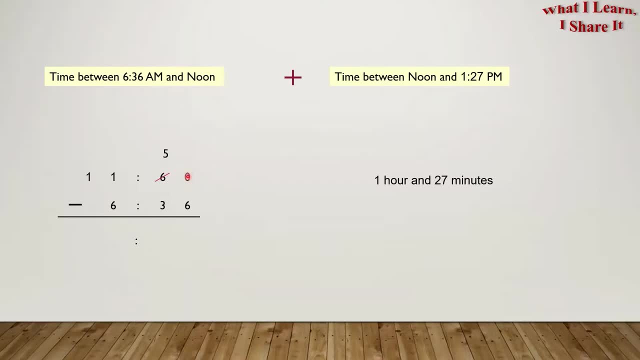 weight will come out to be 10 minutes. The quantity is the higher number, so can we subtract 10 points? The other thing we'll do is we just subtract 10, and we also want to subtract exam 국, we will give 10..